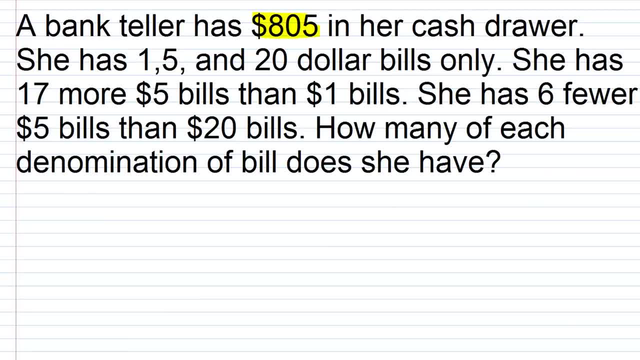 A bank teller has $805, $805 in her cash drawer. She has one, five and twenty dollar bills only. So she has a hundred dollars bills in her cash drawer. She has twenty dollar bills only only. And then here she has 17 more $5 bills than $1 bills. She has six fewer $5 bills. 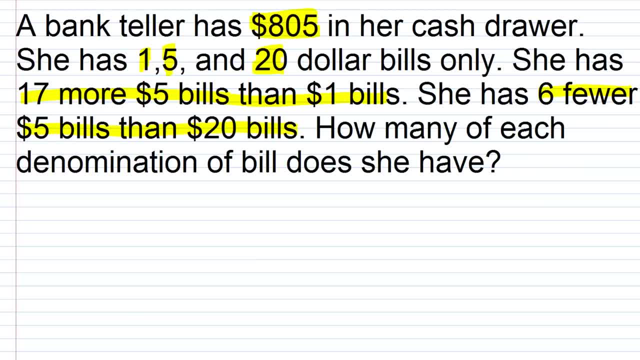 than $20 bills. And then, of course, the main question here is: how many of each denomination of bills does she have? So let's just write out real quick what we're looking to find. We want to know how many $1 bills, $5 bills and $20 bills. So that's what we're trying. 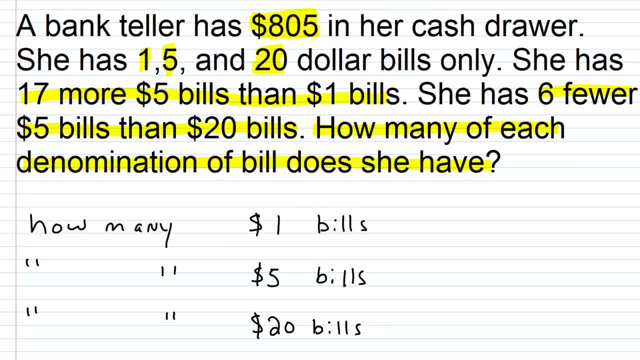 to figure out here. So this will be pretty simple. once we get going here. We want to let x equal one of the amounts here, Either how many $1 bills she has, how many $5 bills she has or how many $20 bills she has When you have a comparison. 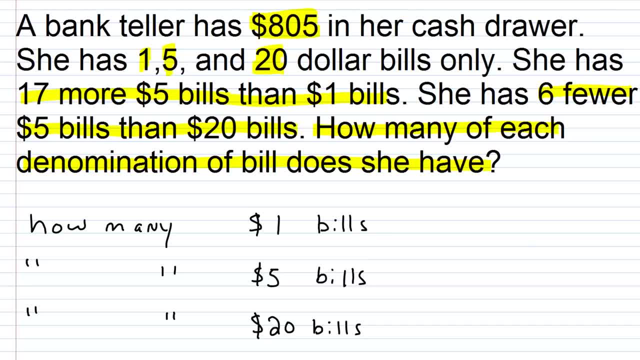 that has three things involved. you usually want to look to see if one of those is involved in both comparisons, And we do have that here, Because here we're told that she has 17 more $5 bills than $1 bills And we're also told that she has six fewer $5 bills than $1 bills. 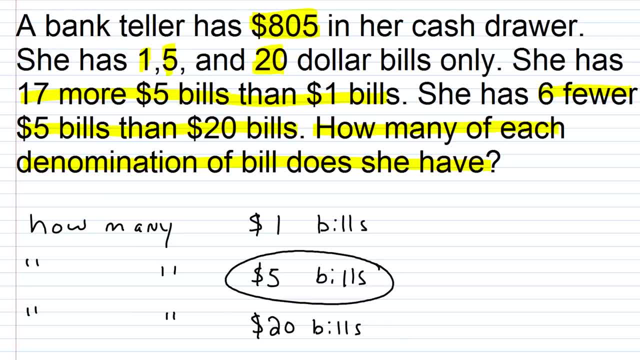 $5 bills than $20 bills. So $5 bills is involved in each comparison. So let's just go ahead and make it easy on ourselves And we'll let x equal the number of $5 bills. Then if we go back and read through the problem, we can base everything on that. 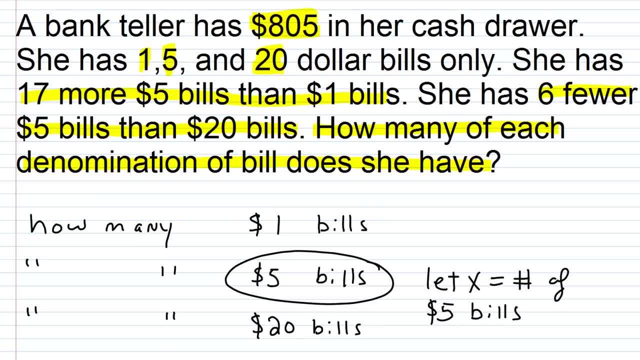 So it's saying that she has 17 more $5 bills than $1 bills. So however many $5 bills she has, she has 17 fewer $1 bills. So then, if x is the number of $5 bills, that means x minus 17. 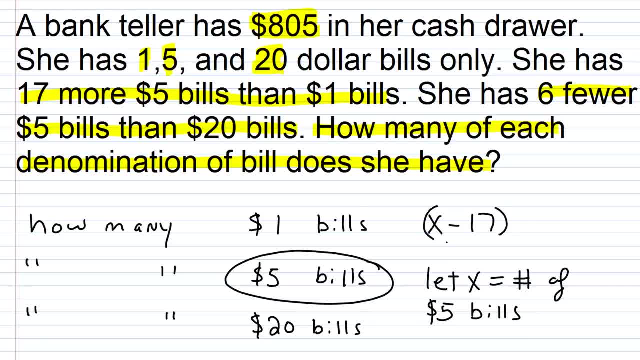 is going to be the number of $1 bills. Okay, and just to reiterate that again, she has 17 more $5 bills than $1 bills. So just flipping that around, she has again 17 fewer $1 bills than $5 bills. Either way you say it's the same. 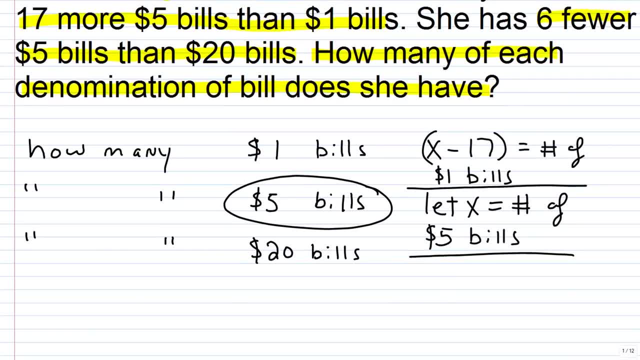 thing. Okay, now let's look at the next comparison. It says she has six fewer $5 bills than $20 bills. So I could really say that the amount of 20s that she has is going to be $5.. So that's. 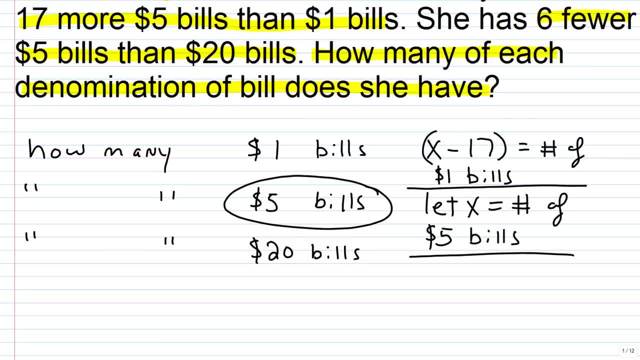 going to be 6 more than the number of 5 she has. So if the number of 5 she has is x, then 6 more than that would be x plus 6.. Okay, so this is going to be equal to the number of $20 bills. 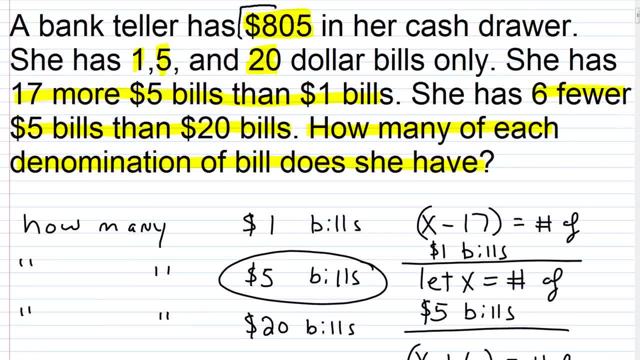 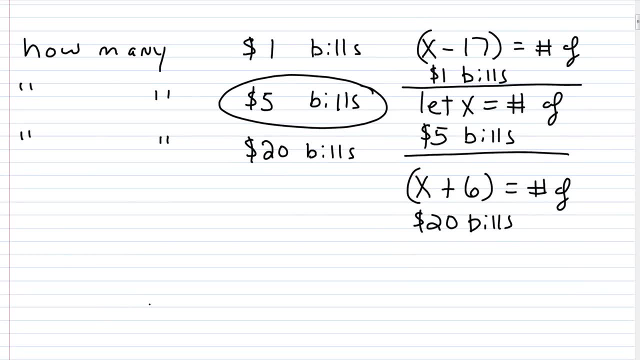 So now we have enough to set up an equation, because this key thing here, this $805 in her cash drawer, it tells us the total amount of all the bills combined. So we can base our equation on that. So let's scroll down here and get a little room. So the number of $1 bills that we 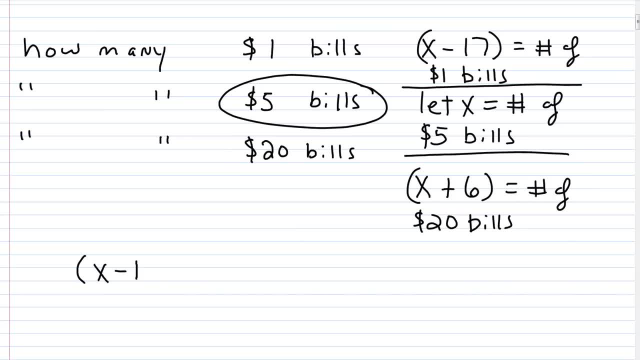 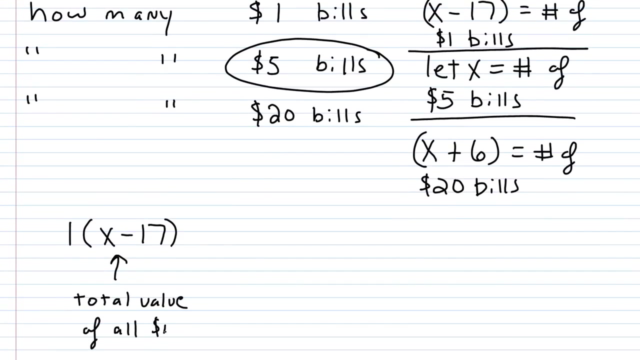 have is x minus 17.. If we multiply that by 1,, which would be the value of each bill, we're going to get the total amount in dollars that we have in ones, So the total value of all the $1 bills. Now we're just going to go through and add this to the total value for all the 5s. 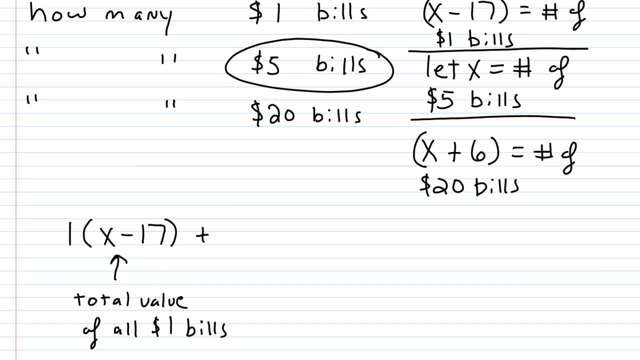 the total value for all the 20s, and we can just set that equal to $805, because that's the total value of all the bills combined. So then we'll have, plus we have, the number of $5 bills, that's x. 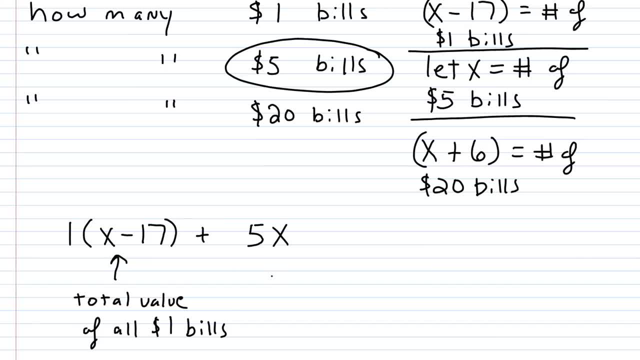 times the value of each bill, which is 5.. Again, this is the total value Of all $5 bills. Then, plus how many 20s do we have? We have x plus 6.. And then times the value of each bill, which is going to be 20.. And again, this is going to be. 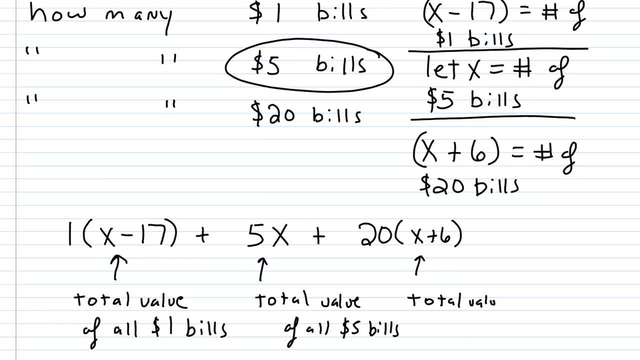 the total value of all $20 bills. Then, when we sum these amounts, we're going to get $805, right, That's what we're told in the problem, So we're going to get $805, right, So we're going to get $805,. 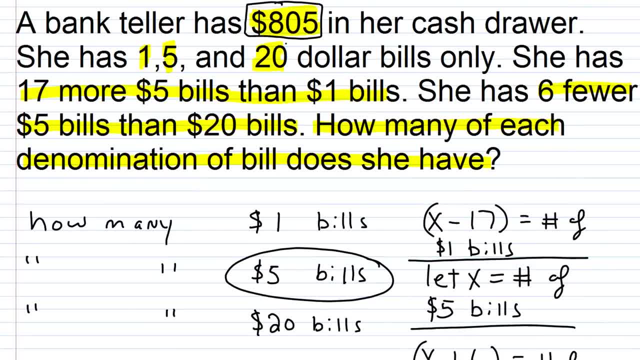 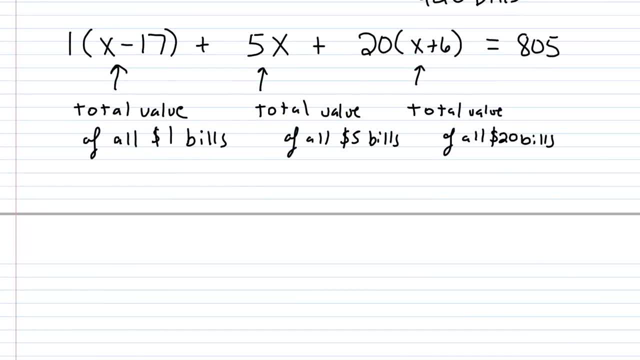 again, a bank teller has $805 in her cash flow, So if we take the total value of all the bills, it's going to equal $805.. Okay, so let's go ahead and solve this equation now And we'll just rewrite it 1 times: x minus 17 is just x minus 17.. And plus 5x, then plus 20 times. 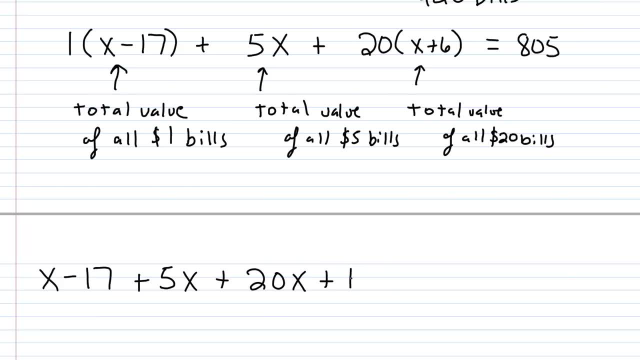 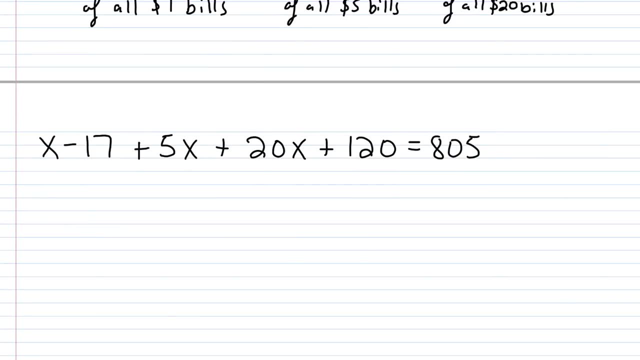 x is 20x plus 20 times 6,, which is 120.. Equals 805.. Okay, so we're going to just combine like terms on the left. here We have x plus 5x plus 20x, that's 26x. Okay, I'm just going to mark these out now because I've used them. 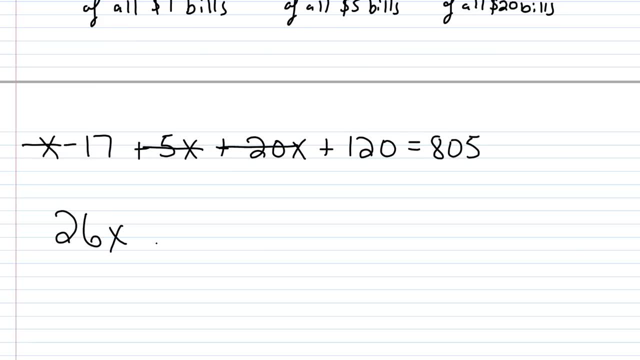 Then I have negative 17 plus 120, that's 103.. Okay, we're going to subtract 103 from both sides of the equation. So we're going to subtract 103 from both sides of the equation. Okay, we're going to subtract 103 from both sides of the equation. 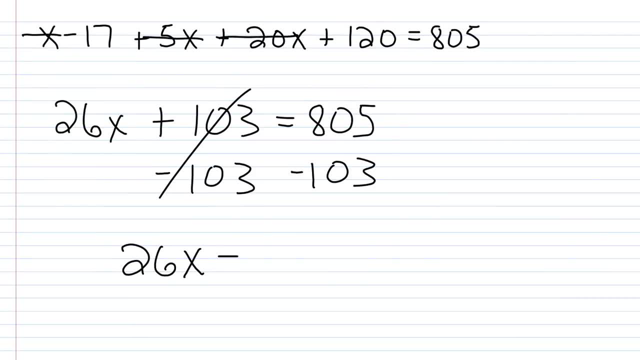 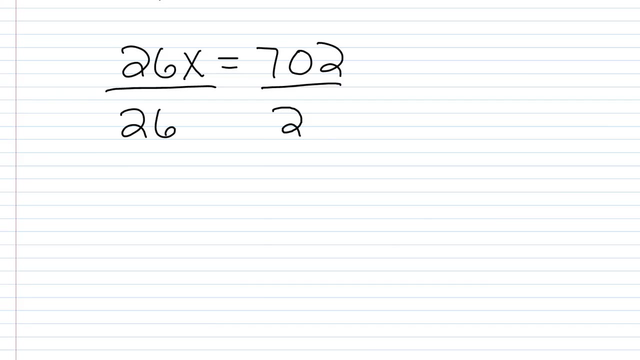 That's gone, You'll have 26x equals 702.. Now to solve for x. we divide both sides of the equation by 26. And we get x equals 27.. And again, we're not done. Yeah, we know, x equals 27.. 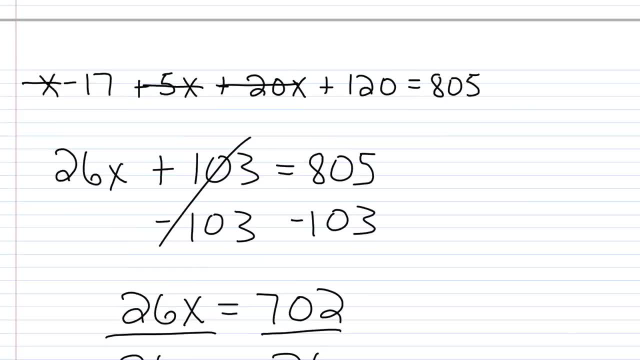 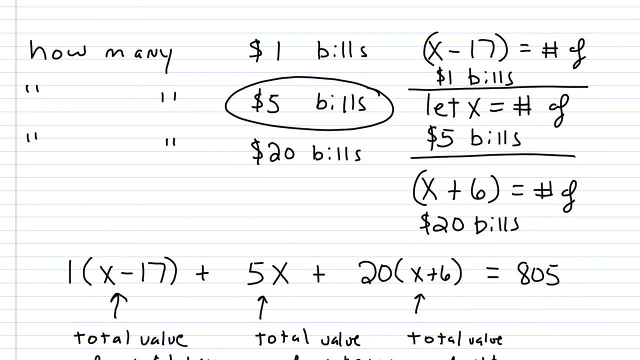 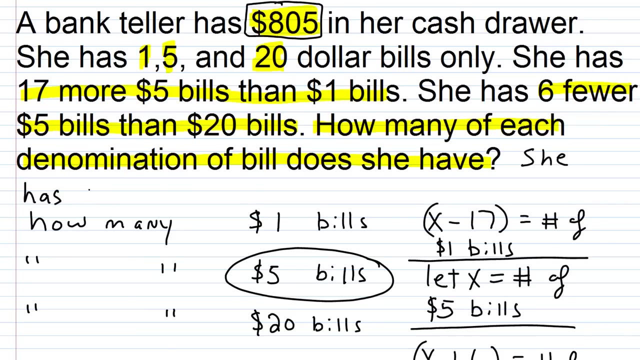 But whenever you're solving a word problem, you have to make sense of it. So we go back up here And we see that x was representing the number of $5 bills. So that means that she has 27 $5 bills. So then, how many 1s does she have? 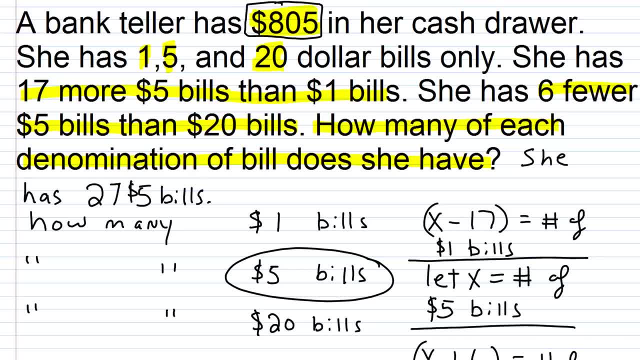 Well, it's x minus 27.. x minus 27.. x minus 27.. So if x is 27,, 27 minus 17 is 10.. That means she's going to have 10 $1 bills. So she has 10 $1 bills. 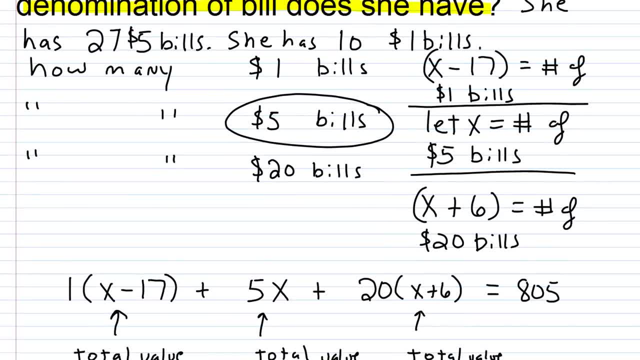 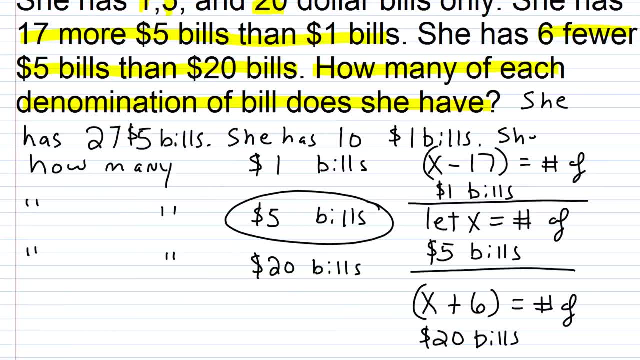 And then how many 20s. We go down here to how many 20s she has. It's x plus 6, so it's 27 plus 6,, that's 33.. So then she also has 33 20 $1 bills. 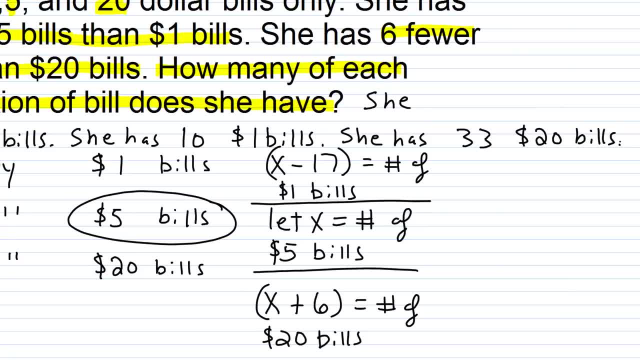 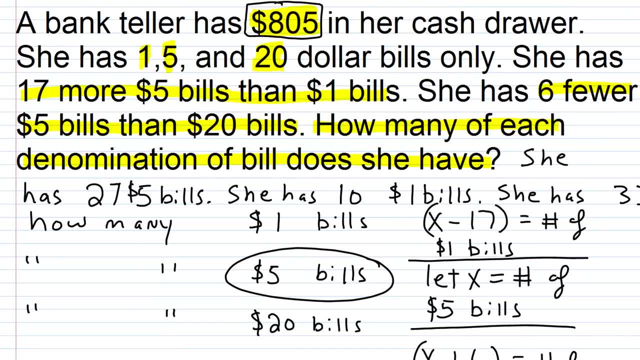 So that would be the answer. Now, to check it, you just verify Again. if we're told in the beginning of the problem that she has $805 in her cash drawer and she only has three different types of bills: she has 1s, 5s and 20s. 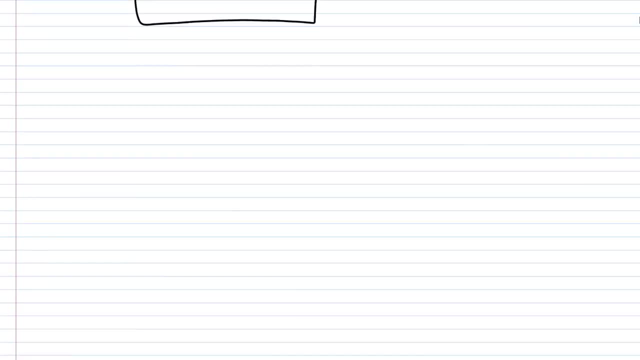 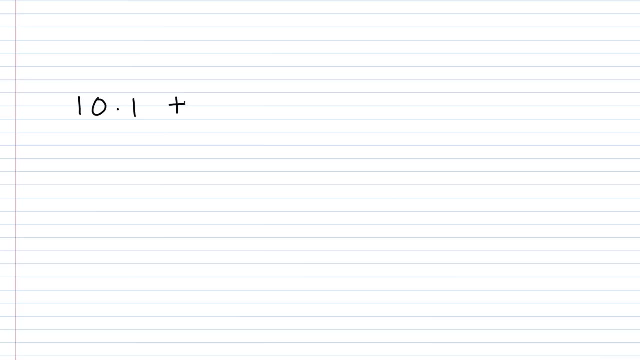 we can go back through and just verify our equation that we set up Again: if she has 10- 1s, so that's 10 times 1, plus, if she has 27- 5s, so that's 27 times 5,. 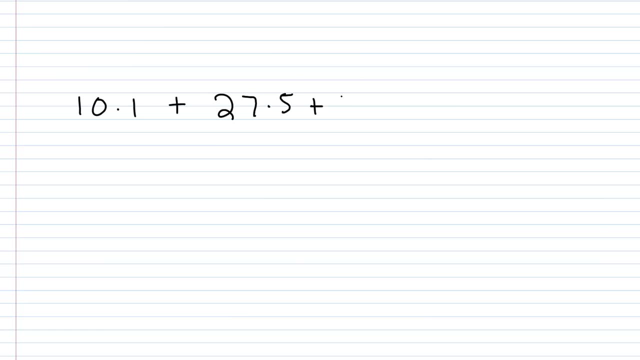 and then she has 33- 20s. so that's 33 times 20,. if we got the correct answer by setting this up, it should equal 805.. 10 times 1 is 10.. 27 times 5 is 135.. 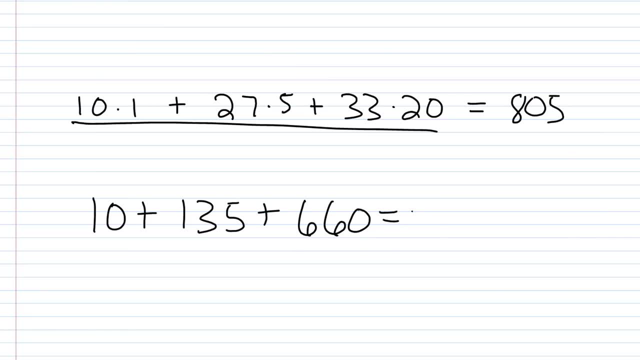 And 33 times 20 is 660.. And then, if we sum these amounts up here, 10 plus 135 is 145.. And then, if we sum these amounts up here and 145 plus 660 is 805.. So everything checks out here. 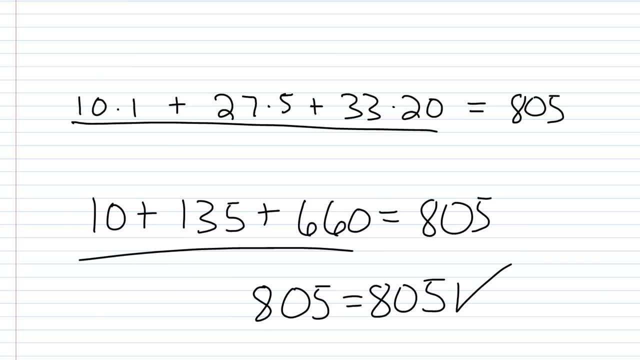 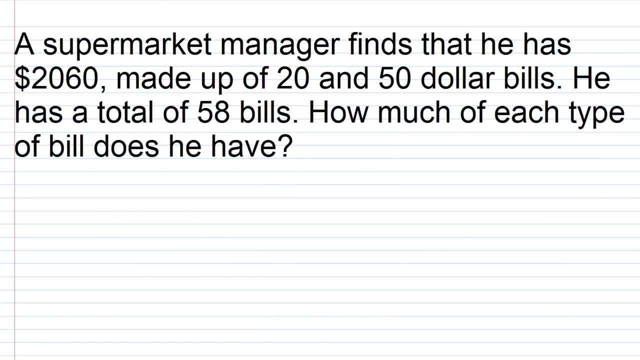 So the teller has 10 1s, she has 27 5s and she has 33 20s. Okay, a supermarket manager finds that he has $2,060 made up of $20 and $50 bills. 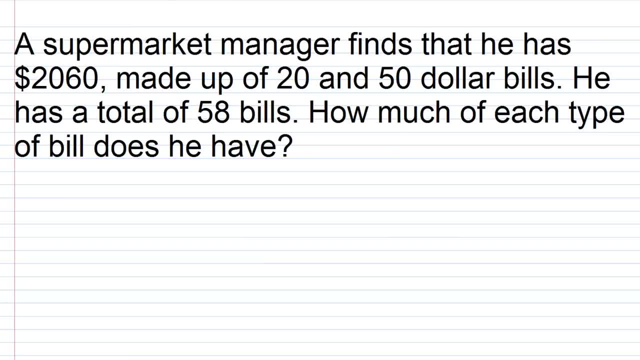 Here's a total of 58 bills. How much of each type of bill does he have? So this is a simple problem here, And basically we're going to solve it kind of in the same way that we solved the first one, but it'll be a little faster. 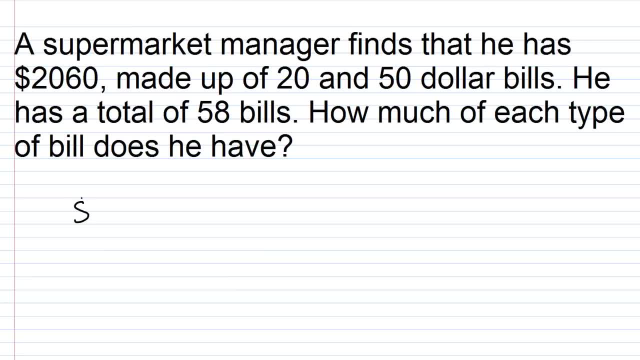 If we know he only has two types of bills- he has $20 bills and he has $50 bills- And the goal here is to find out how much of each type of bill does he have? Well then, we can just start off by just letting x. 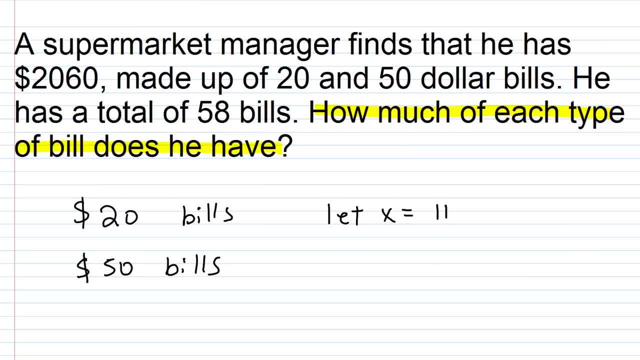 and let x equal the number of $20 bills. So what are we going to have? how are we going to model the $50 bills? Well, if you read closely through this, it tells us that he has a total of 58 bills. 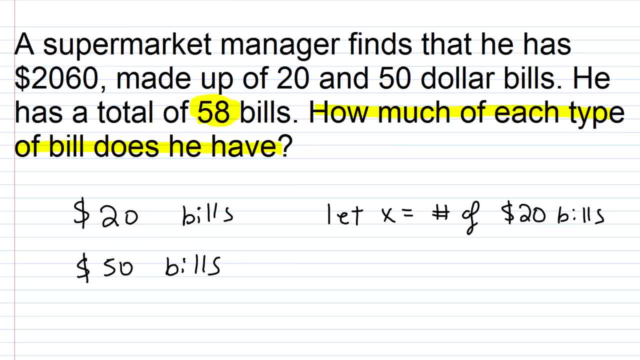 So if he has 58 bills and x is the number of 20s that he has, then 58 minus x, right? 58 subtracting the number of $20 bills that you have is the number of bills that you have. 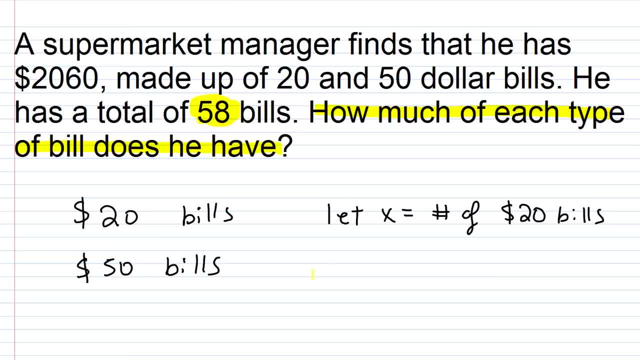 It's going to tell you how many 50s you have, So then. so then, 58 is the total number of bills minus x, which is the number of $20 bills is going to be equal to the number of $50 bills. 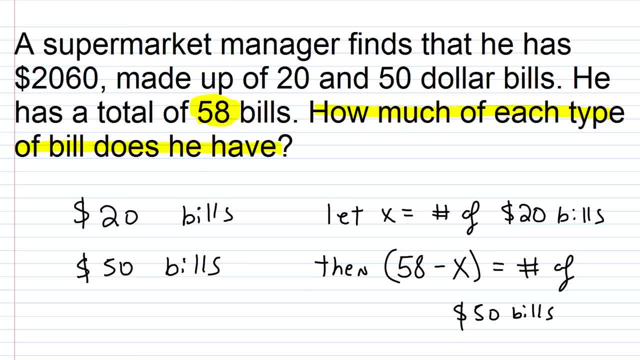 So that's simple enough. So now we've represented the number of $20 bills with x and the number of $50 bills with 58 minus x. So now all we have to do is: we're going to do this. So now we're going to do this. 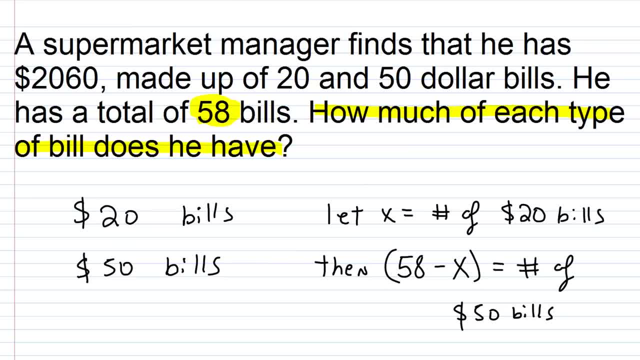 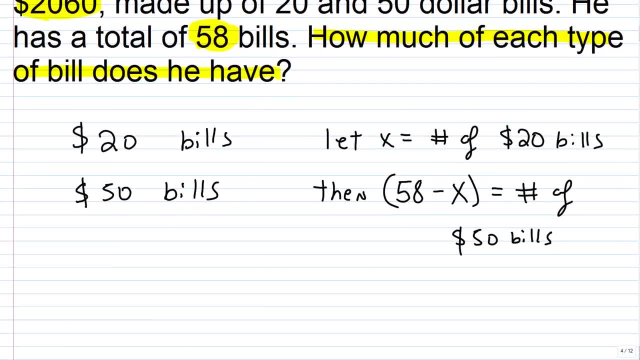 So now all we have to do is just set up an equation. Now the key thing here is that we're told again the value of all the bills here $2,060.. So if we just take the value of all the $20 bills, 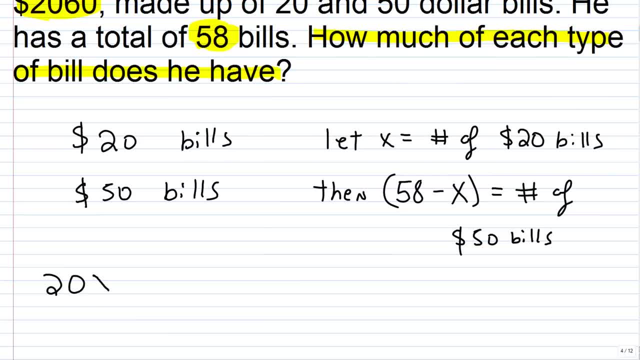 which would be 20,. the value of each bill times x the number of $20 bills, and we add that to the number of $50 bills, which is 58 minus x times the value of each $50 bill, which is 50,. 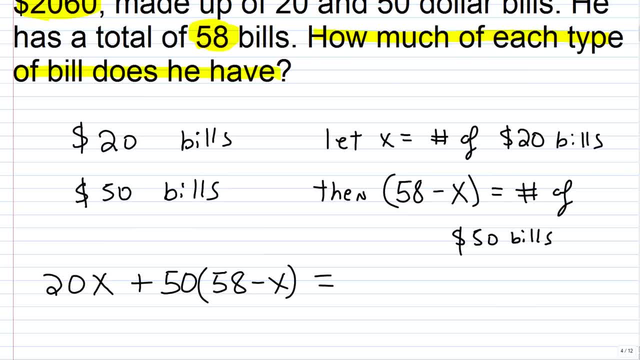 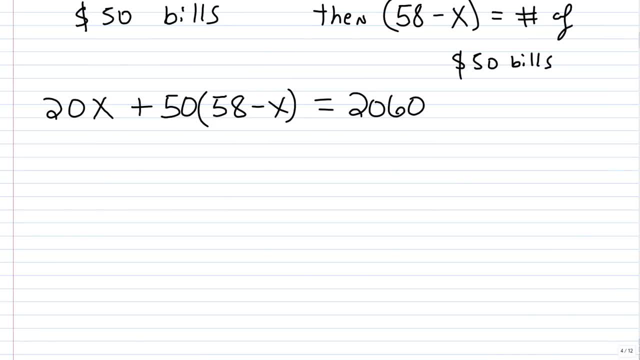 times the value of each $50 bill, which is 50,. This should sum to again this number here: 2,060. So let's go ahead and solve this equation. We'll have 20x plus 50 times 58, That's 2,900. 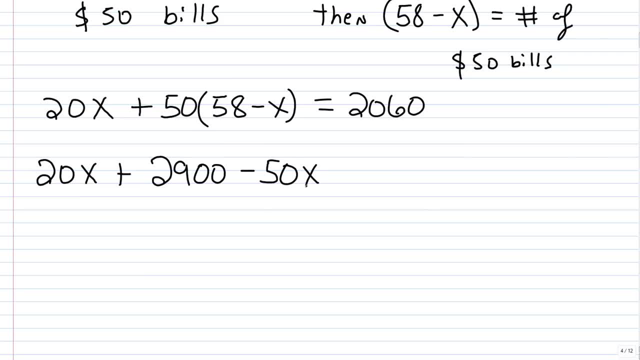 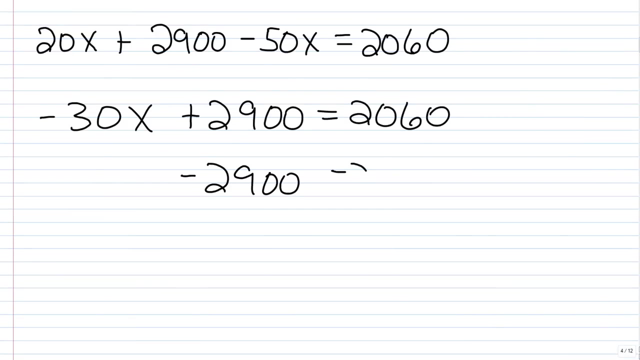 Minus 50 times x Equals 2,060. I'm going to combine like terms here. We'll have negative 30x Plus 2,900 Equals 2,060. Then I'm going to subtract 2,900 from both sides of the equation.